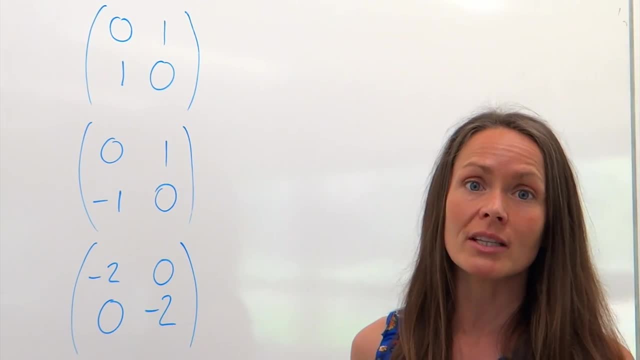 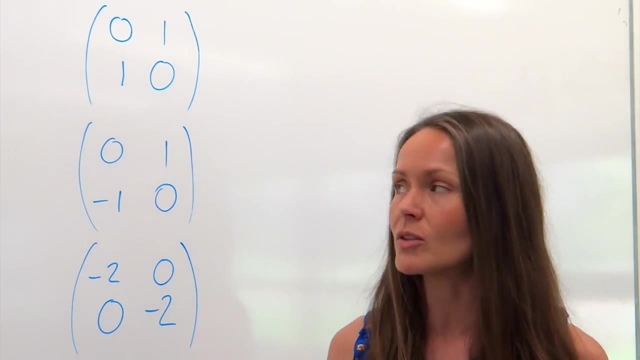 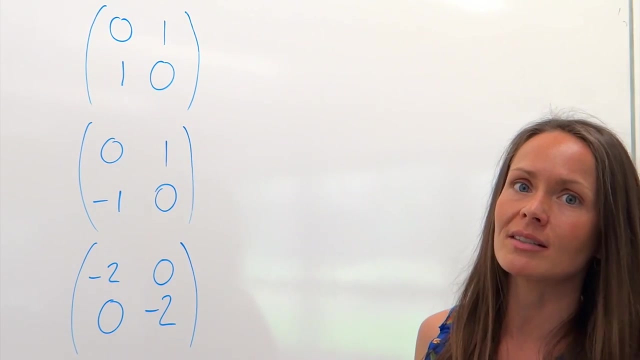 to cover today. these matrices all represent transformations, So transformations could be rotation, reflection or enlargement. So I'm going to show you a method to help you identify what type of transformation this matrix is, for example. So we're going to start by drawing a little axis. 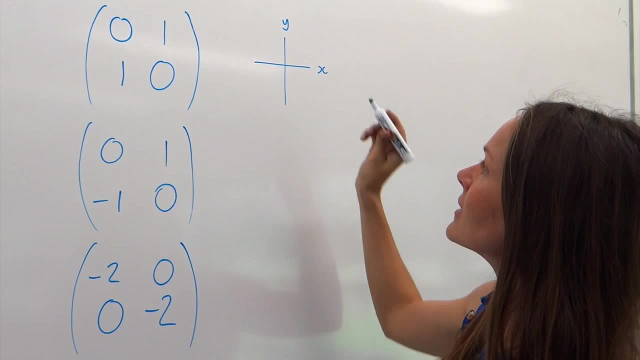 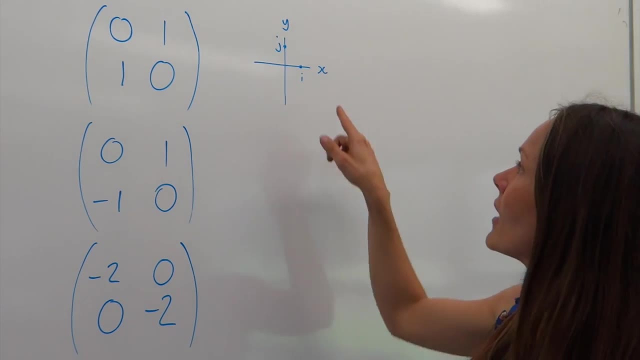 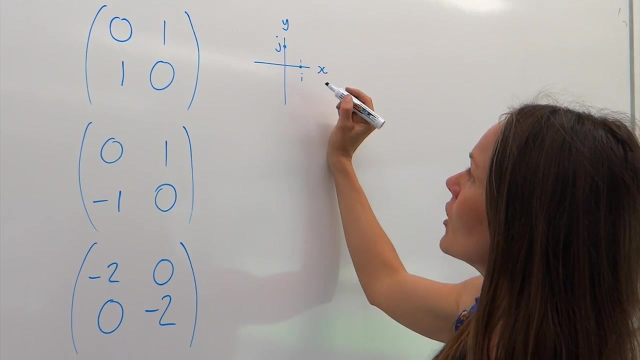 we've got my x-axis here and my y-axis and we're going to use something called base vectors. Now, these are my base vectors- i and j- and they're always positioned in the same place. to start with, i is always one unit along and j is always one unit up. These are the 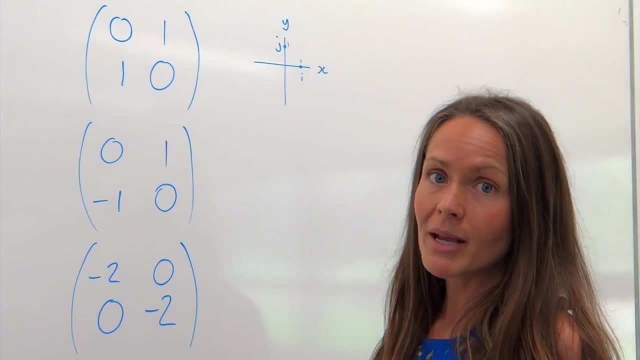 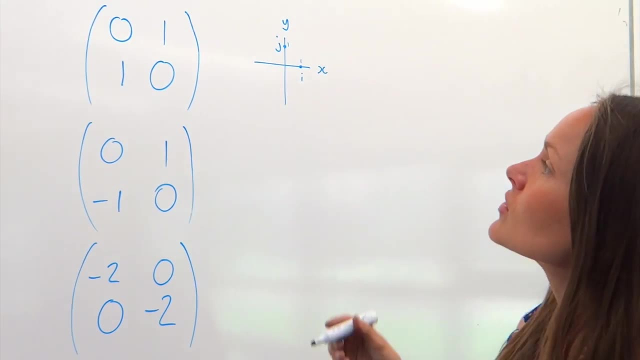 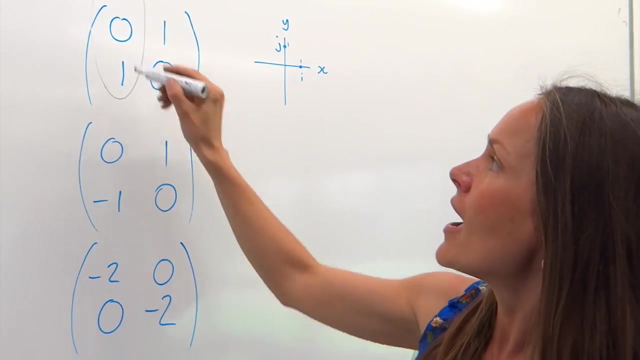 coordinates of i and j after the transformation. so the image of i and j, Because, remember, the object is what you start with and the image is what you end up with. So the coordinates of i-2, so after the transformation, are given here, x being the coordinate on the top and the y 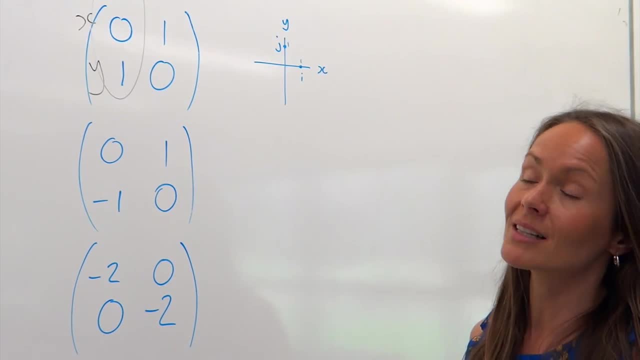 coordinate is the one underneath, So I'm going to plot that on my little sketch. So x is zero, y is one. So i is now up there. so i- is in the same position as j. Now I'm going to do the same. 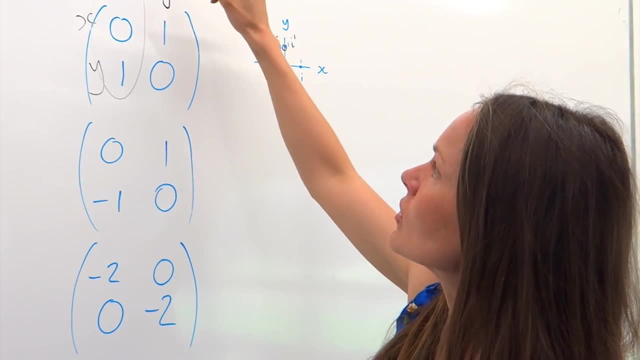 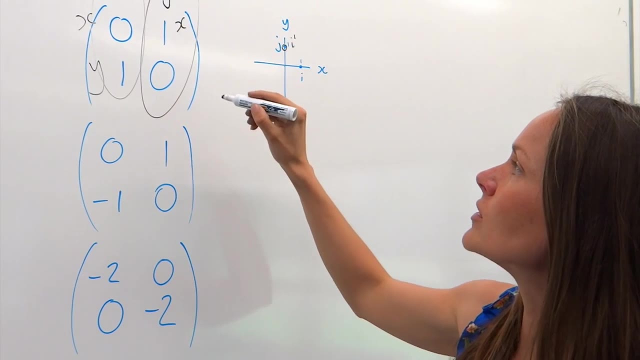 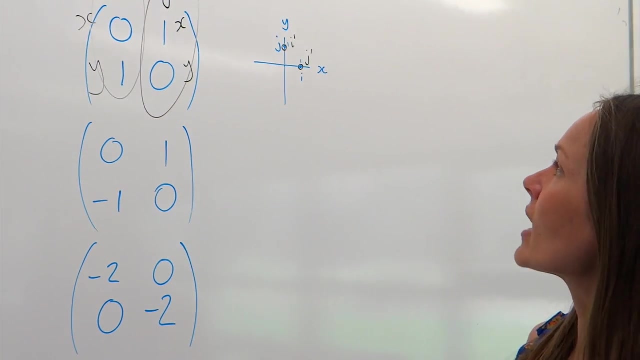 thing with j and I'm going to plot the coordinates of j- So the image of j after the transformation. So this time the x coordinate is one and the y coordinate is zero, which would be there. So i and j have actually swapped places. Now, if you're good at transformations, 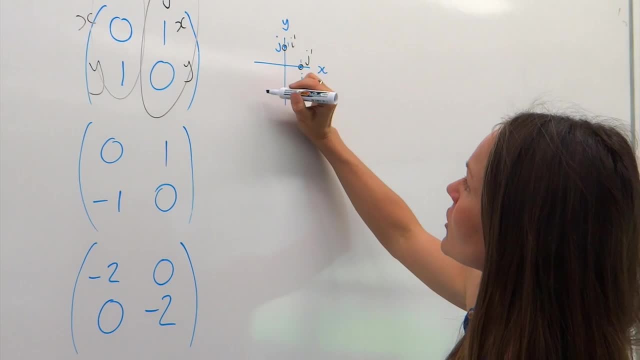 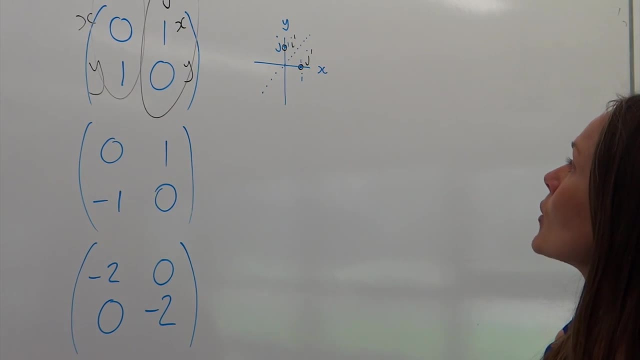 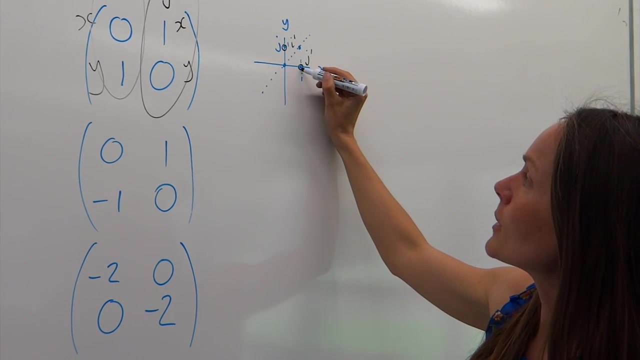 hopefully you've already spotted this one. It's a reflection. You can see that i and j have both been reflected in that line. So we know this point here is zero, zero and this point is one one, Because, remember, here it was in line with one and here it's in line with one. 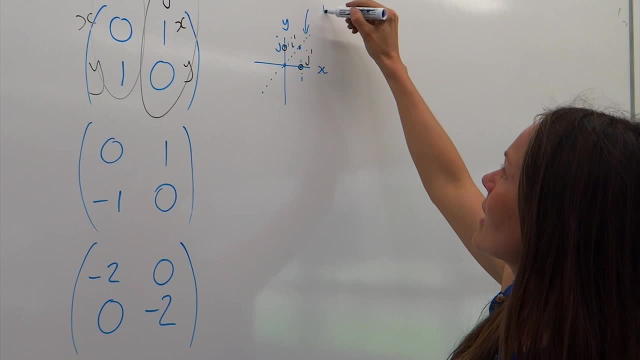 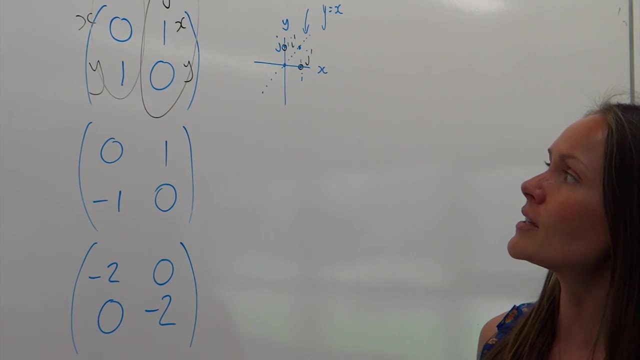 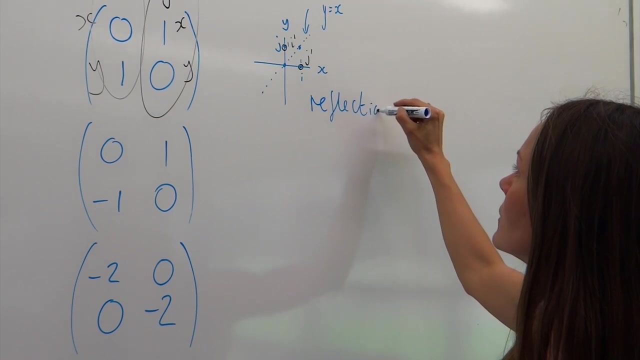 So the equation of that line, that dotted line there is y, equals x. So to get full marks on this question, if it says state the transformation of this matrix, you would have to write the word reflection along with the equation of the mirror line. Okay, so that is how to identify. 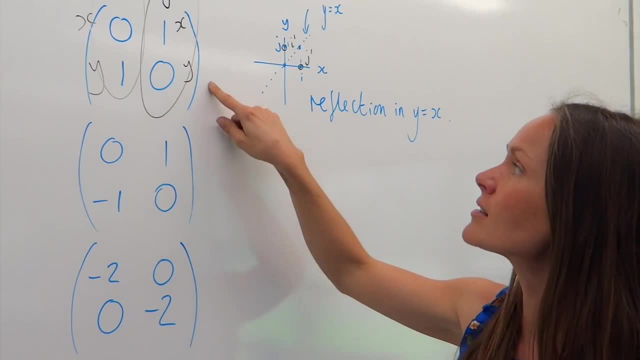 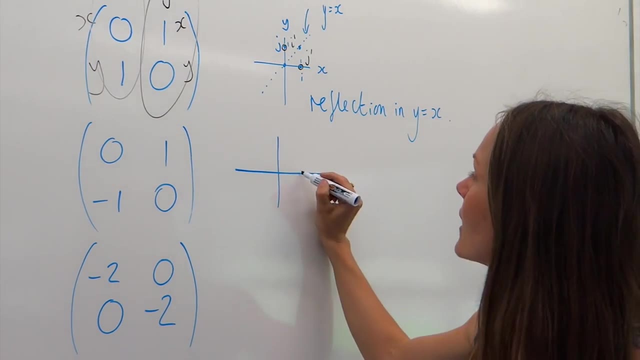 what type of reflection you're going to get. So that's the equation of the mirror line. So that's what type of transformation is given here in the matrix using base vectors. Okay, so on to the next one. Again, I'm going to draw my little diagram and I'm going to show i and j And just 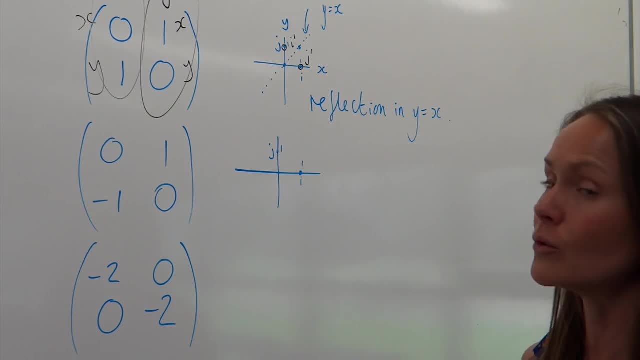 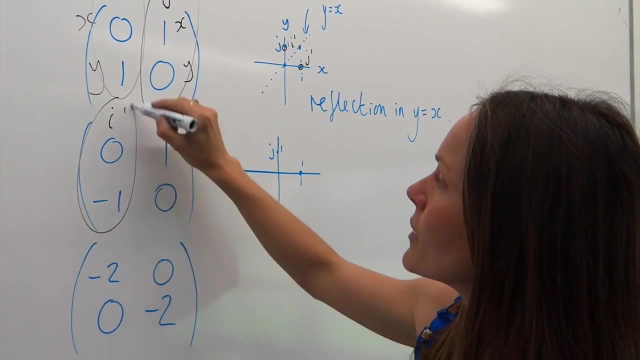 remember, j is always one unit up and i is always one unit along. So, just like in the previous example, i dash is given by this column here. So these are the coordinates of i dash. So this is the x coordinate and this is the y coordinate. So that would be. 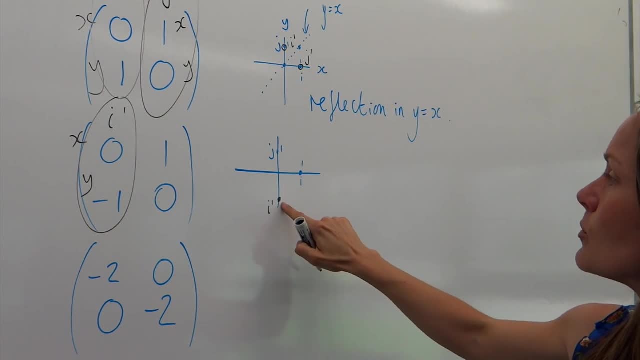 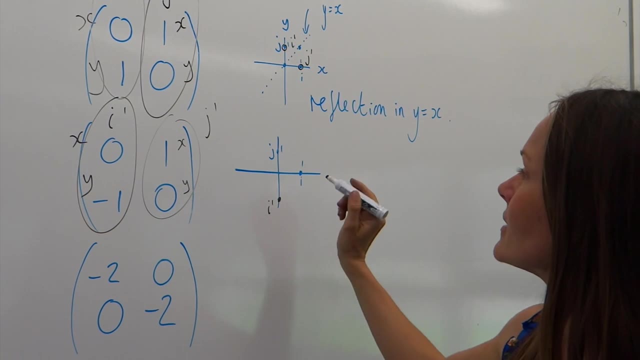 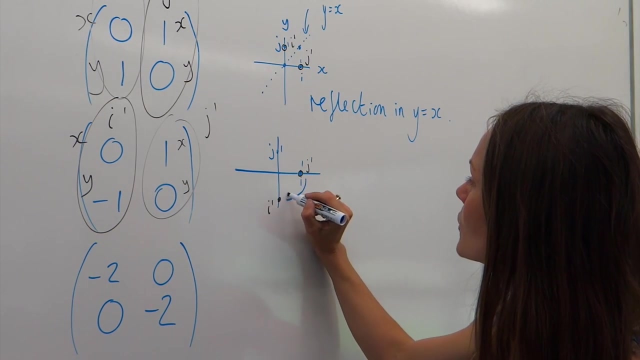 here. Okay, so i dash has moved to here. Now j is at: x equals one, y is zero, which is where i used to be. So on this one, i has moved to here and j has moved to here Now that I've drawn those arrows. 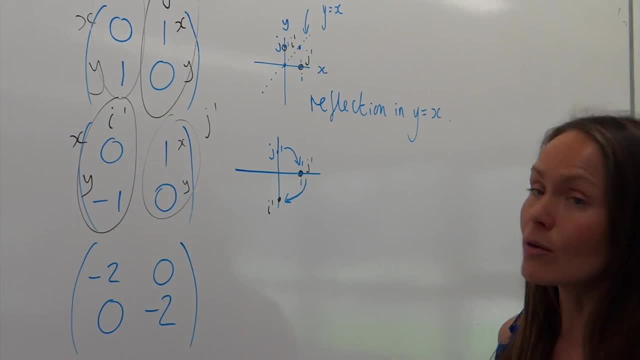 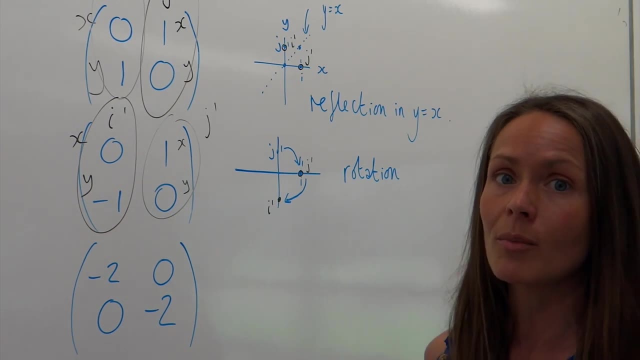 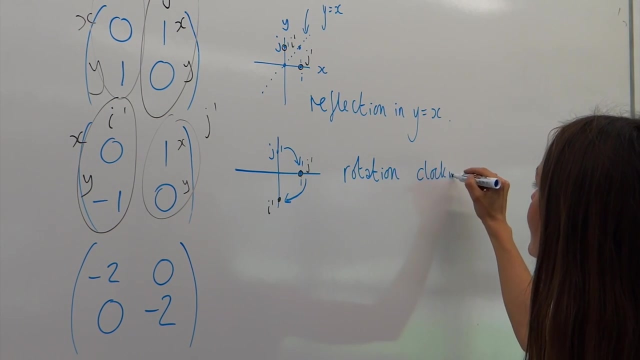 in. you can probably guess which type of transformation this is. It's a rotation. Okay, so that will get you one mark. But we can't just write rotation. We have to describe the transformation fully. So it's rotated clockwise and it's rotated. 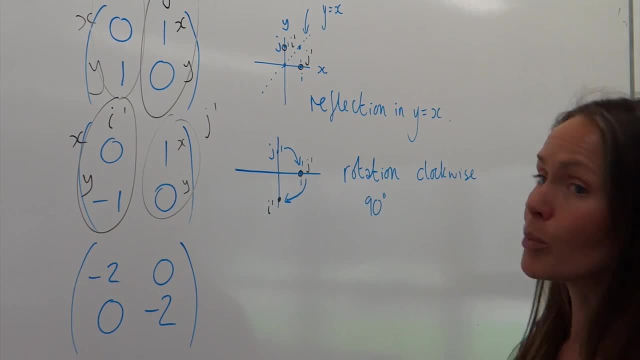 90 degrees And the center point of the rotation is the origin. It's turned around that center origin point. So you also need to write center origin or center zero zero. They're the same thing. So you have to give all of that information. Okay, if you're asked to describe the transformation, 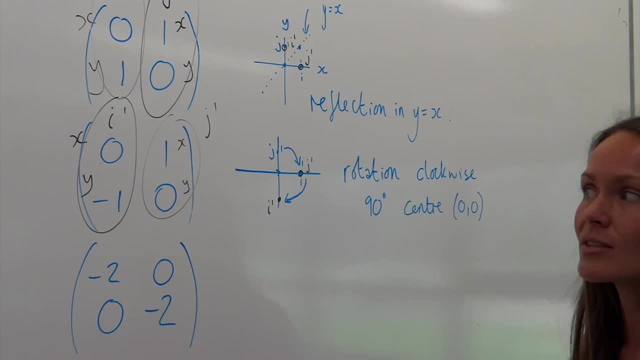 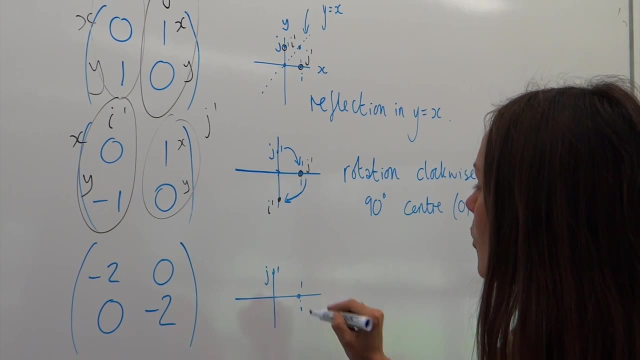 to it. Rotation clockwise: 90 degrees center: zero, zero. Now onto the last one. Same thing again. Find your i and j. Remember one unit up, one unit along. Now i dash has the coordinates of x is. 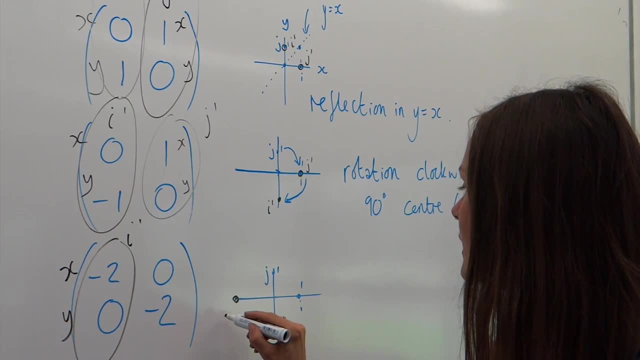 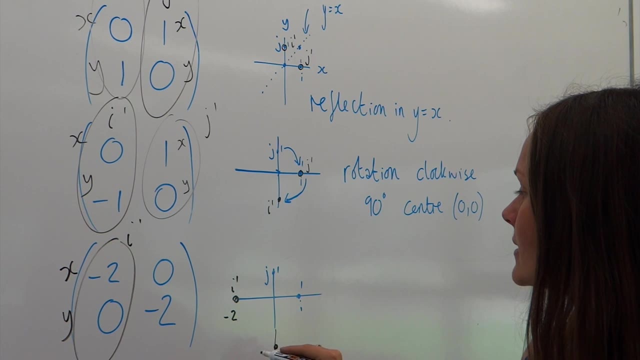 minus two, y is zero. So that would be over here. Okay, so that's i dash And j dash is all the way down there. It's at minus two. Okay, so that's i dash And j dash is all the way down there, It's at.